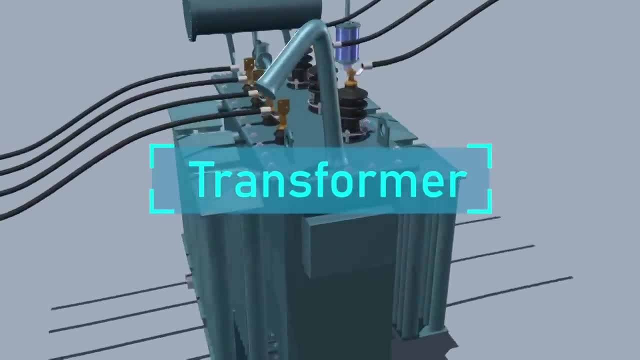 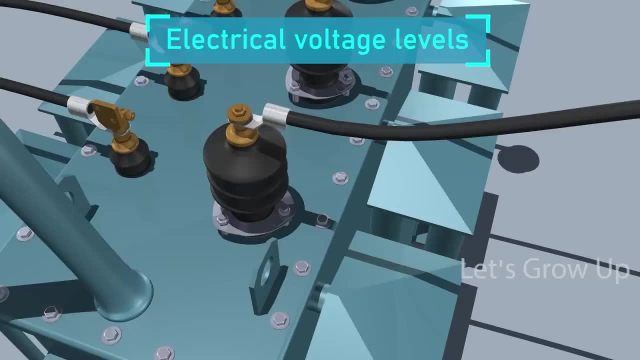 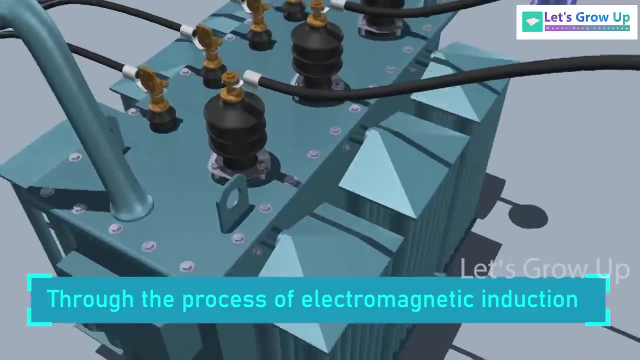 Hi, hope you have seen this transformer. Sometimes it could be a small or big size. A transformer is a passive electrical device that transfers electrical voltage levels from one circuit to another through the process of electromagnetic induction. It is mostly used to increase the voltage levels between circuits, which are called step-up. 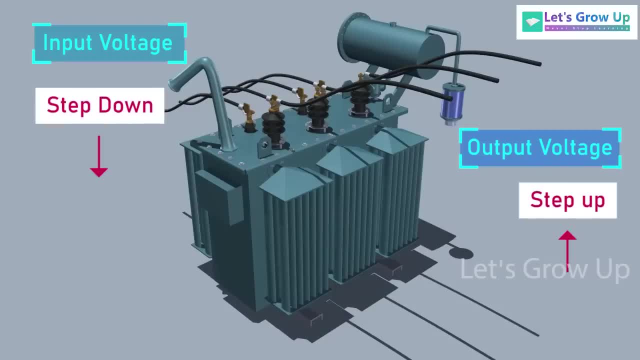 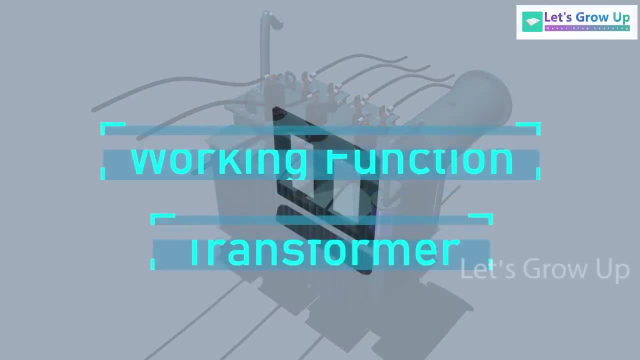 or decrease the voltage, which is called step-down transformer. Today, this video going to explain the working function of the transformer. Let's start with the main parts of the transformer. The core is the main part and it is called the heart of the transformer. 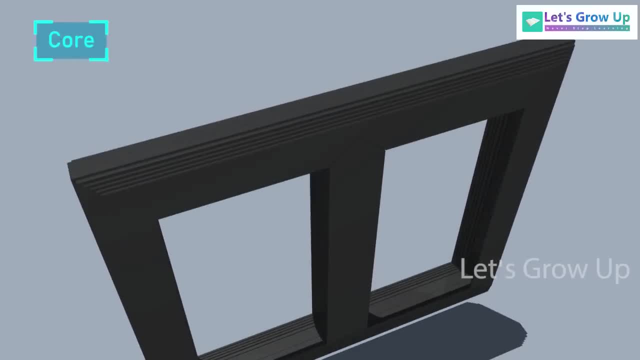 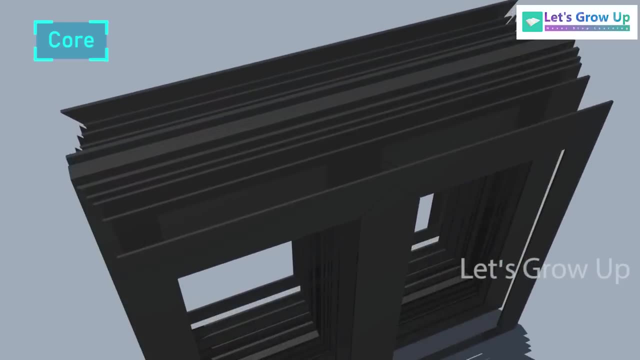 The core is made up of iron or silicon, steel or ferromagnetic materials. It is thin metal strips and lamination insulated by a coat of varnishes or papers. The core of the three-phase transformer consists of three limbs in the same. 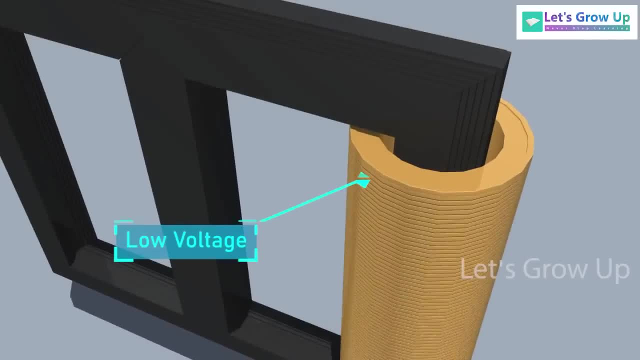 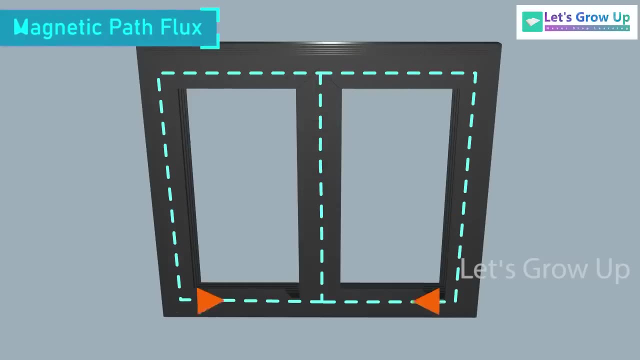 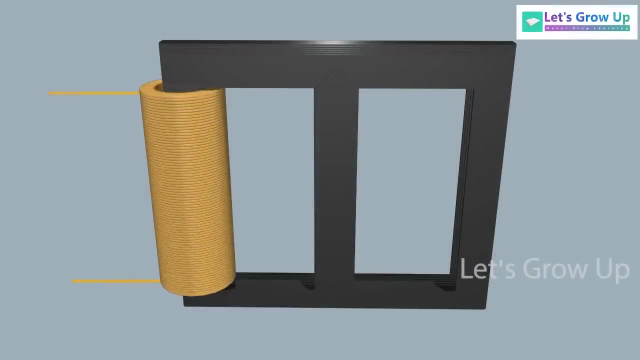 platform And each limb carries both low-voltage LV winding and high-voltage HV winding. The core is provides a magnetic path flux around the core. The first winding is also known as a coil, When it is supplied by an alternating electrical source. 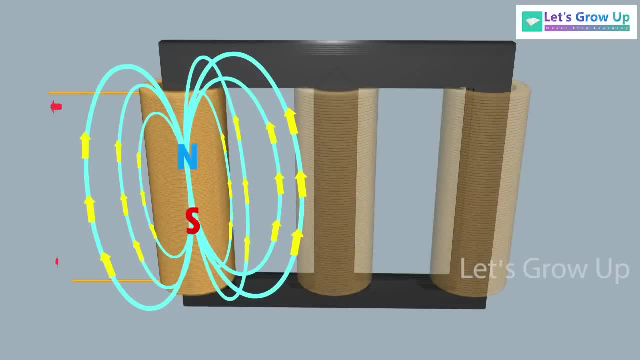 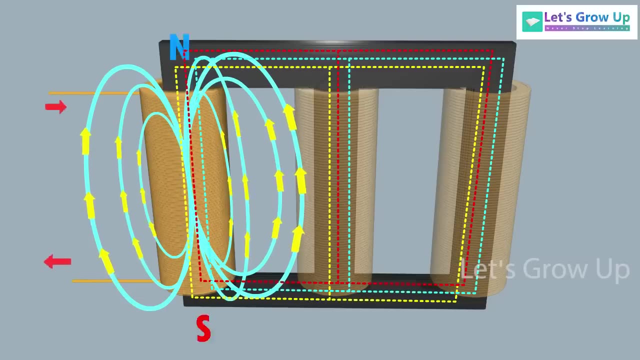 The alternating current through the winding produces a continually changing and alternating flux surrounding it. If another winding is supplied by an alternating electrical source, some portion of this alternating flux will link with the second winding, As this flux is continually changing the amplitude and direction. 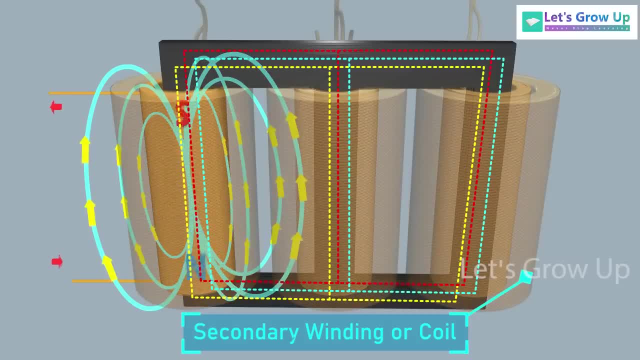 there must be a changing flux linkage in the secondary winding or coil. According to Faraday's law of electromagnetic induction, there will be an EMF induced in the second winding. If the circuit of this secondary winding is closed, then a current will flow through it. 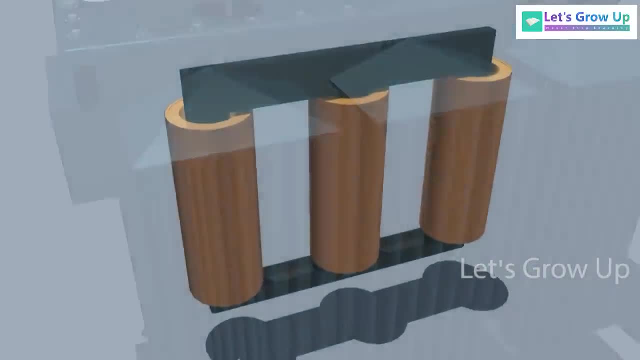 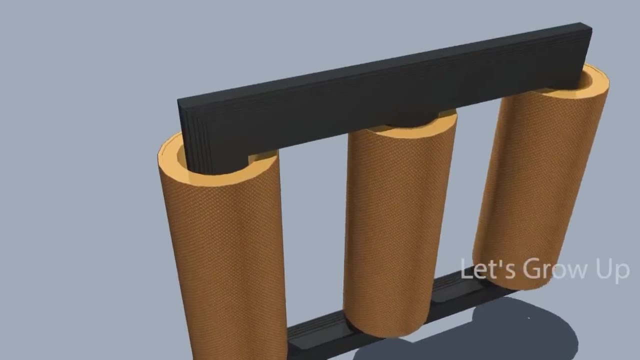 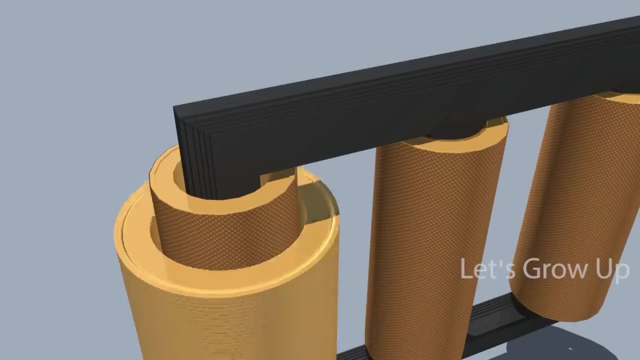 This is the basic working principle of a transformer. The winding which receives electrical power from the source is known as the primary winding. The winding which gives the desired output voltage due to mutual induction is commonly known as the secondary winding. Here, if the number of secondary coil turns is greater than the number of turns primary.